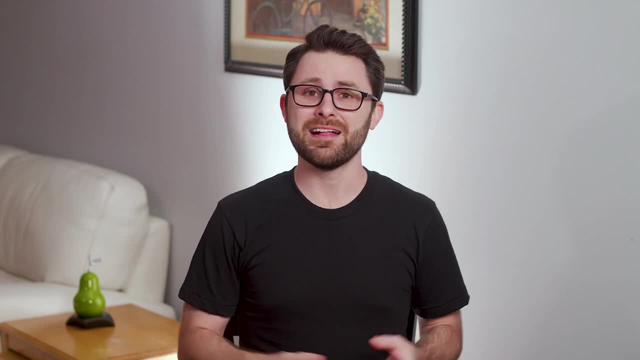 of student loans, credit cards and car loans. Then Dave asks this question: what's the secret to getting out of debt? Nine times out of 10, the response is budgeting. If there's one thing you take away from watching this video, it's the importance of creating a 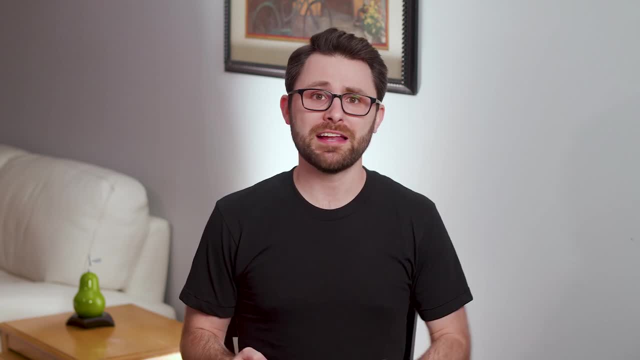 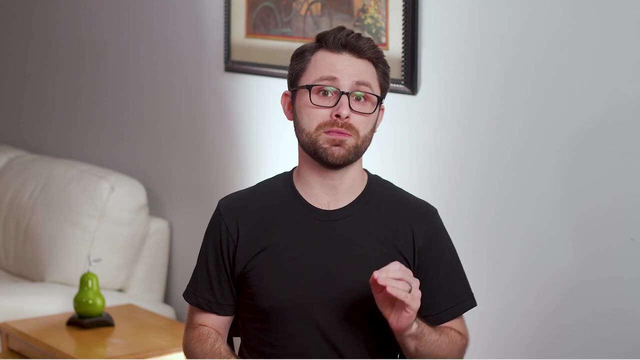 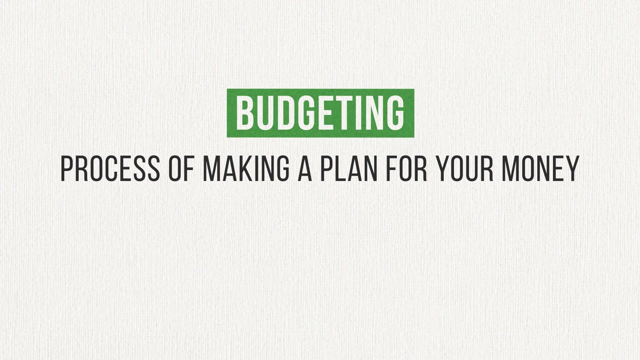 budget, Because if you understand how to create a budget and you take the time to do so on a regular basis, there is no doubt in my mind that you will become successful with money. Budgeting is the process of laying out a plan for your money before it comes in or goes out. You're predicting how. 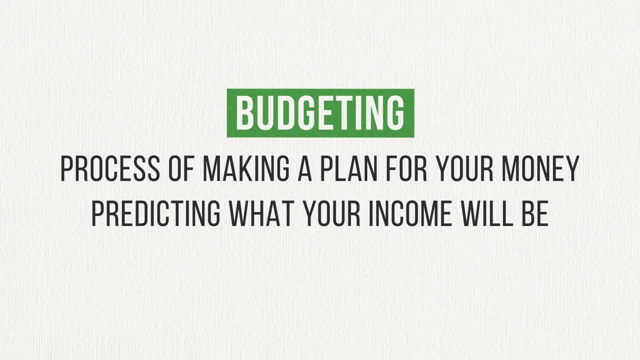 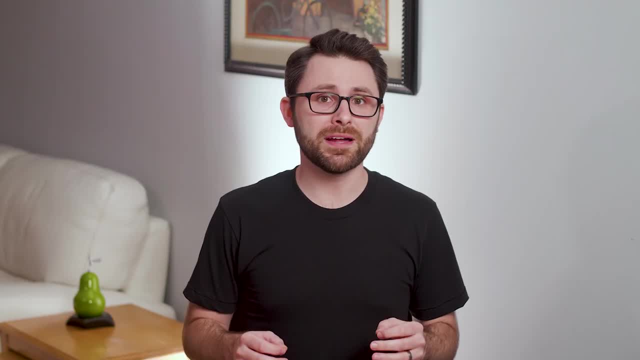 much income you're going to have in a particular time period- usually a month- and then you're deciding how you're going to use that income. The reason so many people struggle with money is that they don't take the time to make a plan for their money. They don't pay attention to how much they're. 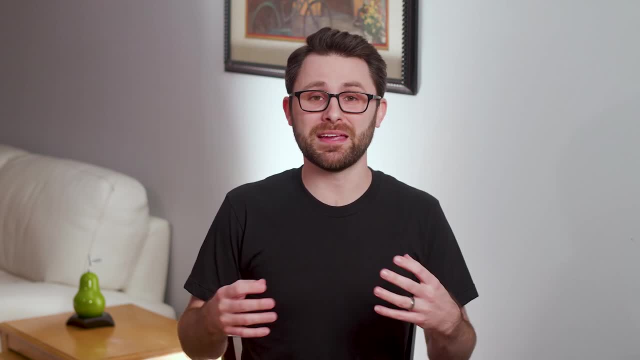 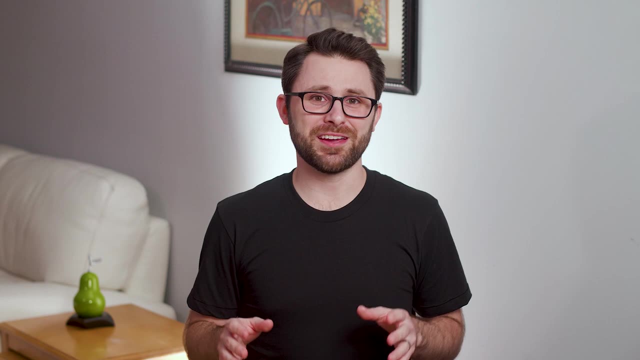 spending, and then they end up spending more money than they have coming in. It's easy to see how this creates a problem. There are no shortage of budgeting apps out there, but I find the easiest way to create a budget is with a spreadsheet. At the beginning of each month, I spend 30 minutes. 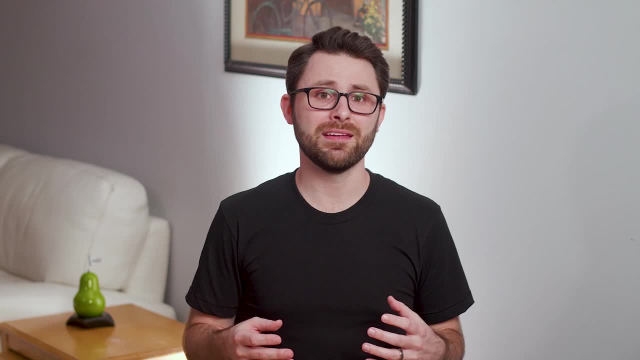 to an hour calculating how much money I expect to have coming in and then laying down a plan for how I'm going to do my spending. I give every dollar an assignment before it even hits my bank account. This allows me to easily make decisions about my spending If it's not something I planned. 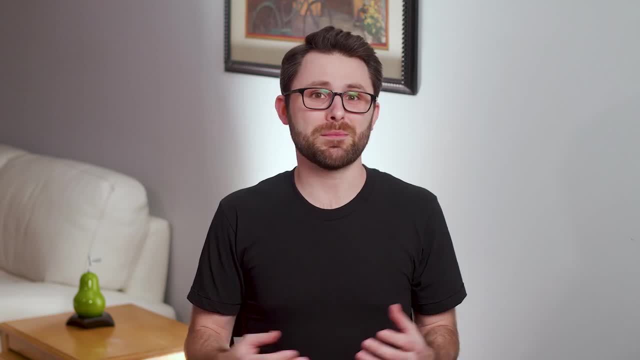 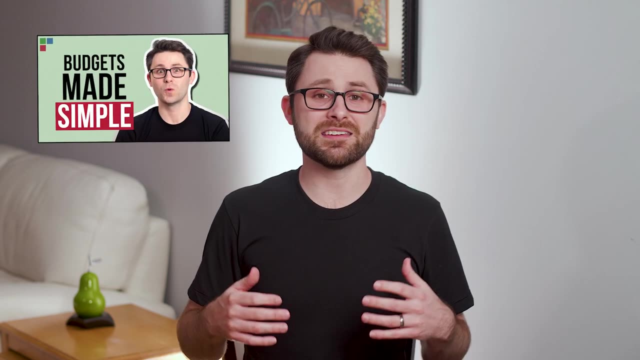 in advance to spend my money on. it's not something I spend my money on. If you want to see the details of how I create a budget, I made a video where I go in-depth and take you through the entire process, And if you're a college student, I made a more specific video tailored to the income. 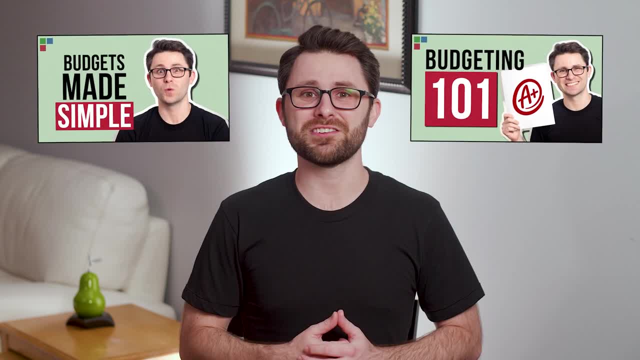 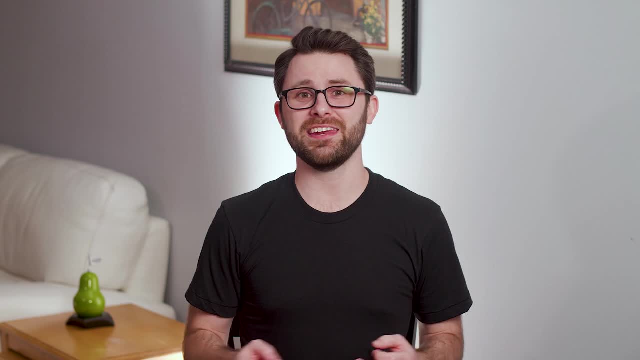 sources you might have while you're in college. Links to both are down below. Topic number two is insurance. Let's say you're walking down a set of stairs at home on a rainy day, You slip and fall and wind up with a broken ankle. You'll need to go to the emergency room. get some x-rays done, have surgery to ensure it heals up properly, get a special boot for walking and attend physical therapy twice a week for three months. All that medical treatment is not going to be cheap. Thankfully, if you've got health insurance that'll pay for the majority of it On a basic 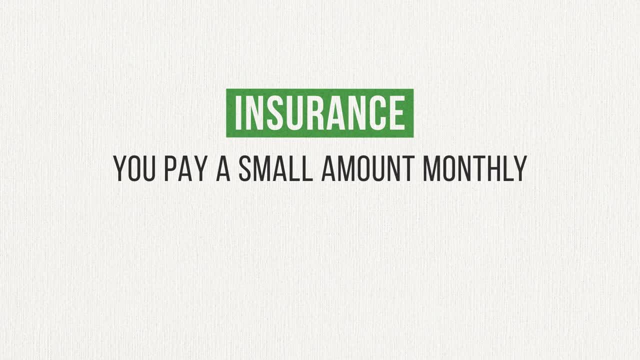 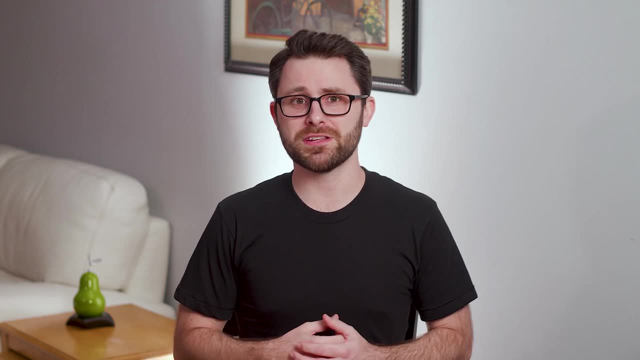 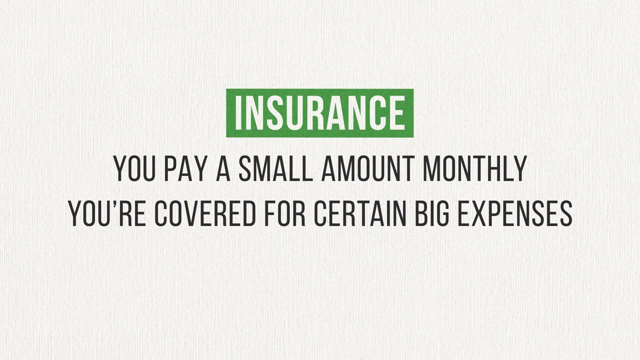 level insurance is something you pay a relatively small amount of money for on a monthly basis. In this example maybe it's a few hundred dollars per month for health insurance. Then if something unexpected and expensive happens, you're only responsible for a small portion of the bill. 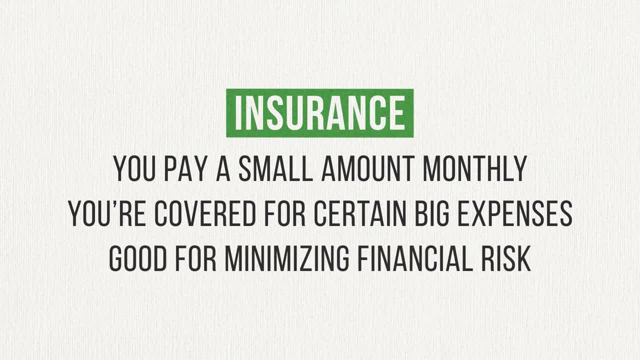 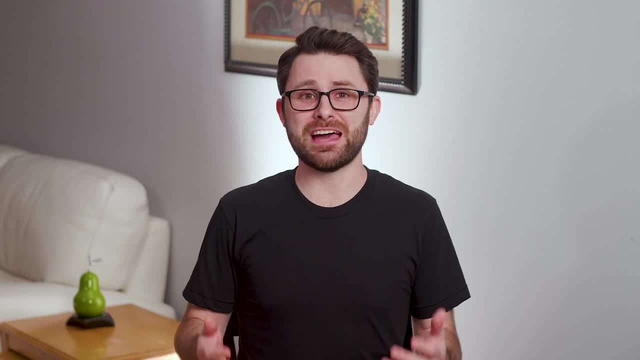 In the case of a broken ankle that requires surgery, this could be the difference between it costing you $1,000 and $30,000.. Most people don't have tens of thousands of dollars just lying around, so they choose to pay a few hundred a month for a health insurance plan That way. if something comes up, they're not financially ruined. If you're in high school, chances are you've already got health insurance and maybe even car insurance through your parents. So while your needs should be taken care of for the time being, they'll become your responsibility as you move on. 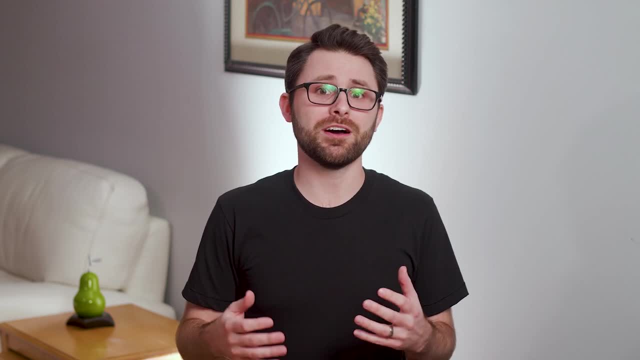 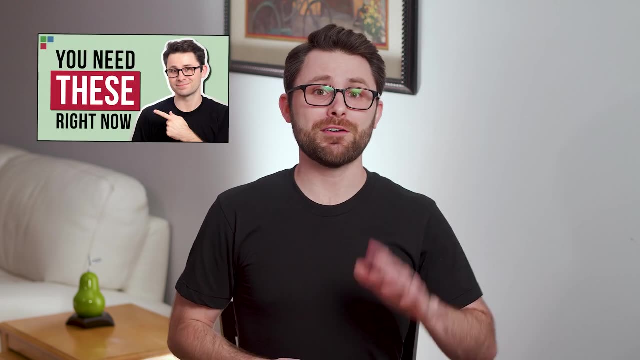 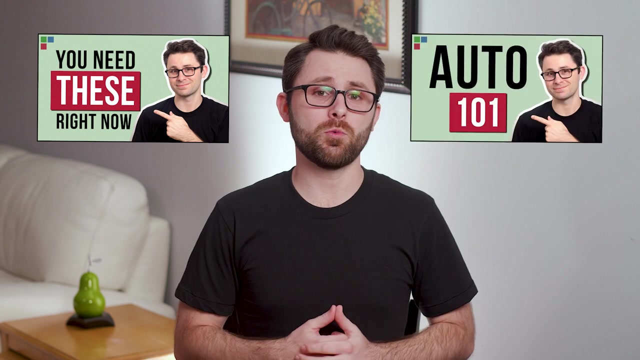 into adulthood, It will become important to have a good understanding of the types of insurance available and how they work. If you're interested, I made a video about the five different types of insurance you'll probably need to purchase before you're 30 years old. I also made a video where I 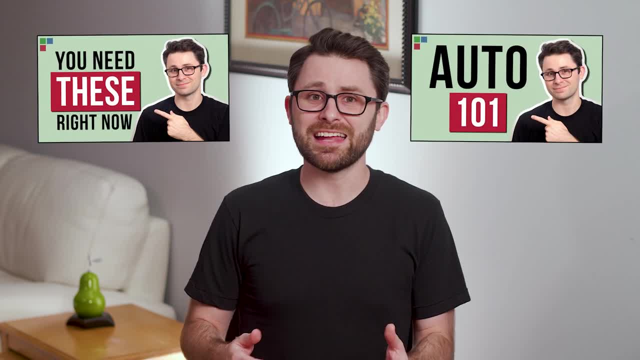 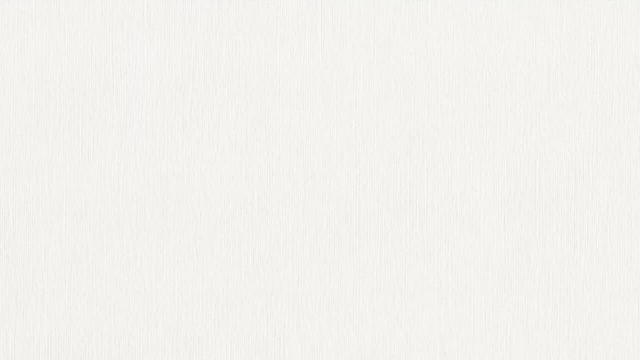 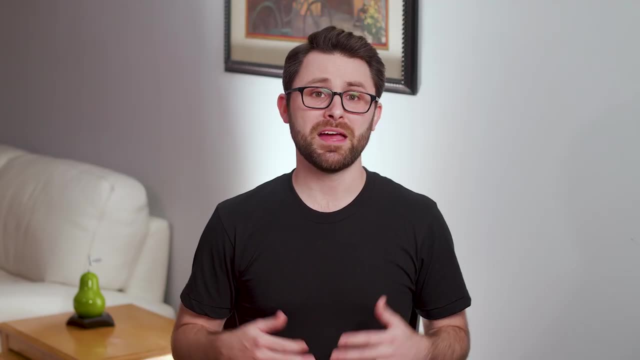 go in-depth into every aspect of car insurance and give you my recommendations for how much coverage you need. Links to both of those videos are down below. Topic number three is interest. Think about the process of renting a car. You walk into Enterprise, pay a rental fee and you get to take. 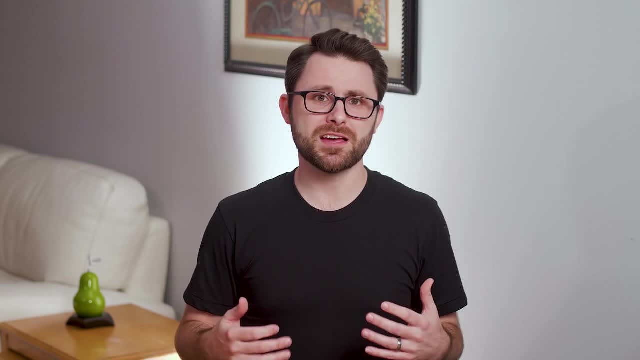 one of their vehicles for a few days. When your rental period is up, you bring the car back. Interest is like a rental fee, but instead of borrowing a car, you're borrowing money. Anytime, you borrow money to buy something, be it a student loan, to pay for your college tuition, a car loan. 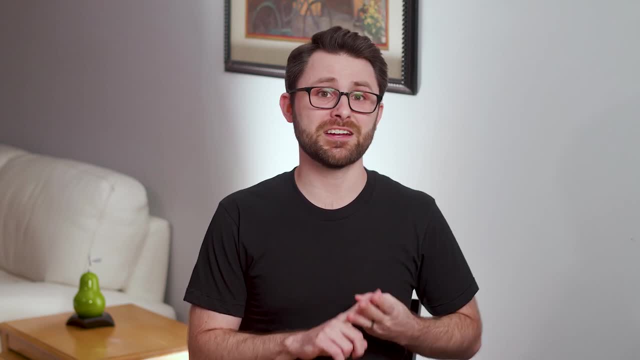 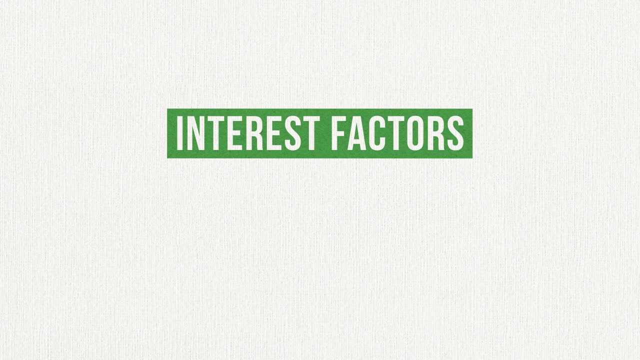 to buy a new Mustang, or even a swipe of the old credit card to buy a chicken sandwich at Popeye's, you're going to be stuck paying interest. The amount of interest you're going to be stuck paying depends on two factors: The amount of money you borrowed but haven't paid back. 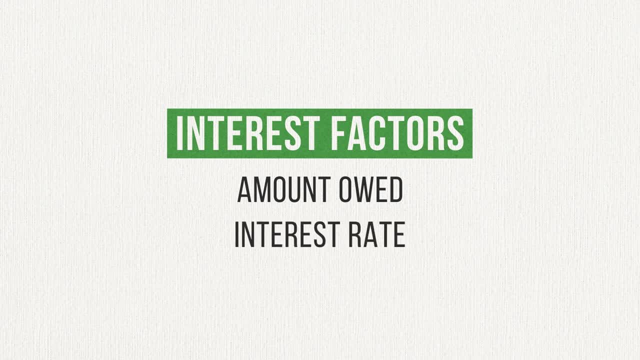 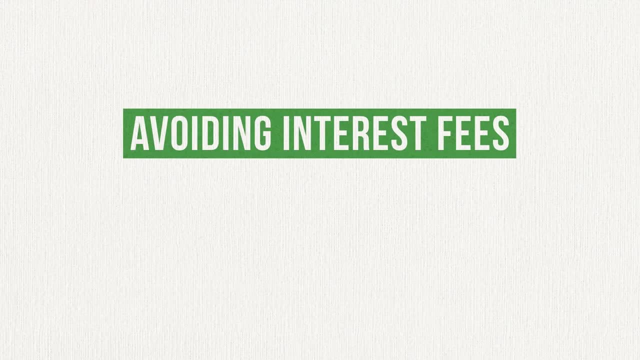 and the interest rate. The more money you have left to pay back and the higher the interest rate you have on the loan, the more interest you're going to pay. So if you want to avoid paying a ton of interest fees, you wanna limit the amount you borrow and 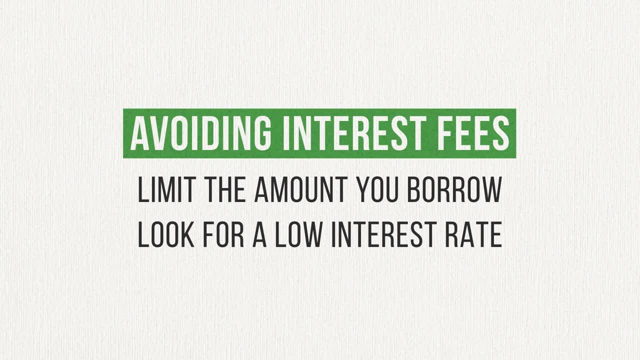 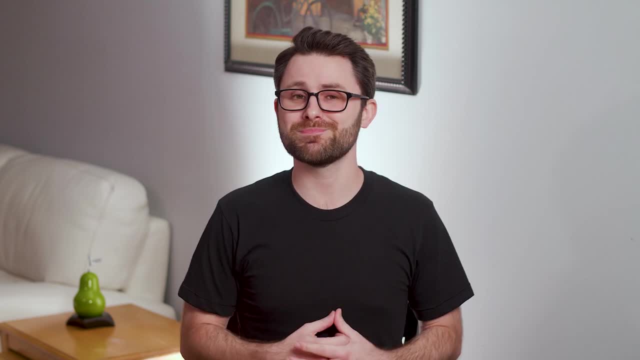 sure you get a low interest rate when you do. I spent my entire college career not paying attention to how much I was borrowing and what the interest rates were on my student loans. Later on, I ended up having to pay nearly $10,000 per year in interest fees alone- not 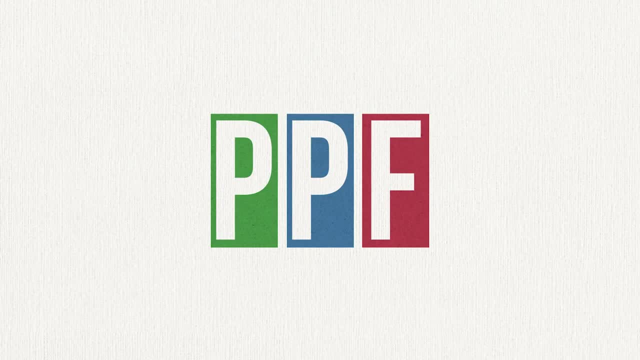 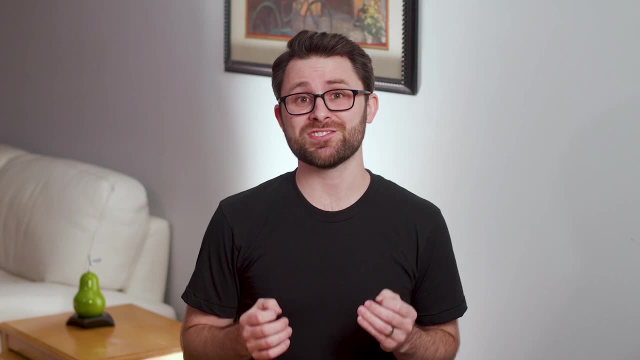 counting the amount of student loans I had to repay. When you're in debt, like I was, interest really sucks. But when you're investing, interest will become your best friend. The other aspect of interest you need to know about is called compounding. Let's say you put $100 into an investment that pays you 10% interest per year. 10% of $100 is $10.. So after a year you have $110 in that investment. 10% of $110 is $11.. 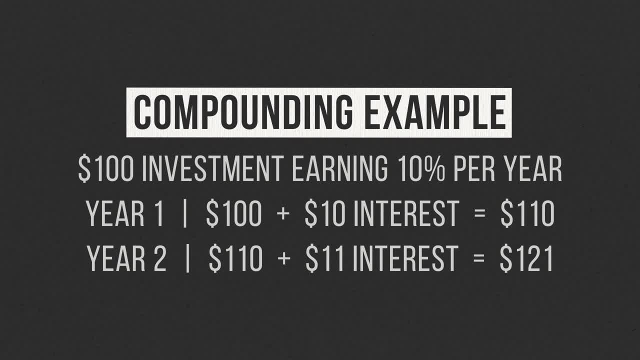 So after year two you have $121 in that investment. The reason you earned $11 in year two instead of $10 is because you earned $11.. That extra dollar in year two is interest on the interest you earned in year one also. 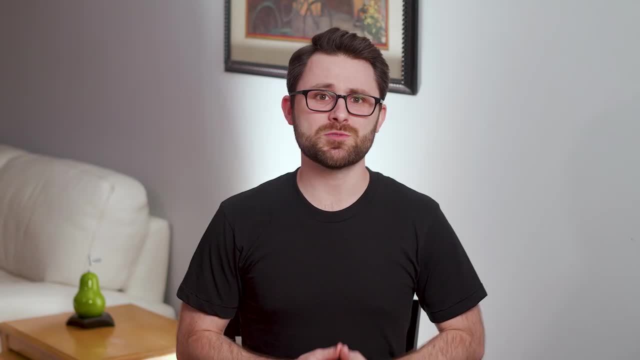 known as compound interest. Compound interest is one of the most powerful wealth-building tools available to you, and understanding how it works is a major key to becoming wealthy. If you'd like to learn more about interest, I made videos where I explore the topics of: 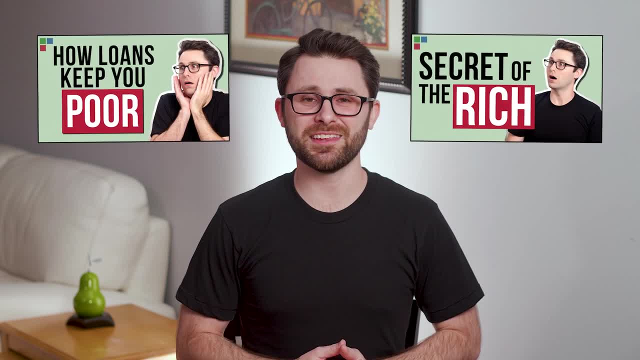 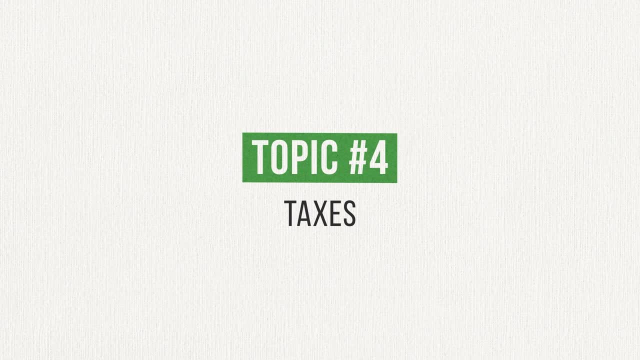 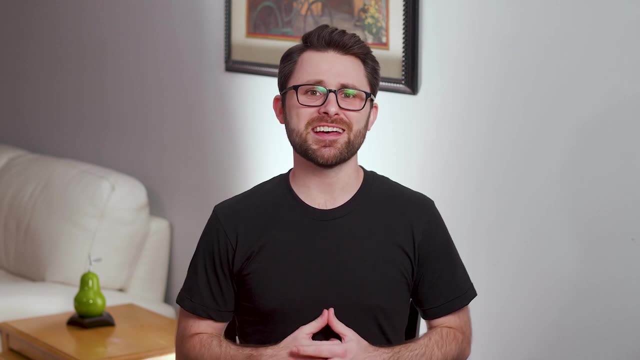 interest on student loans. The links to both of those are down below. Topic number four is taxes. Imagine ordering a pizza and having it delivered. You pay the price on the menu and tip the delivery driver when he shows up at your door. You get inside and open up the pizza box only to find that two of the eight slices 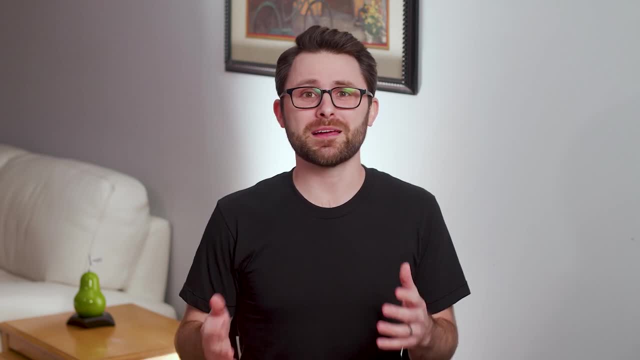 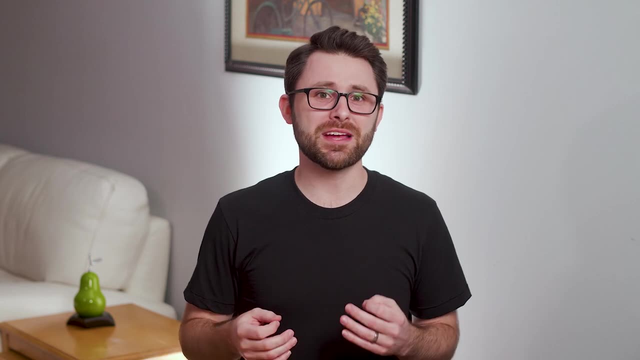 are missing, What gives? Well, if your paycheck was like a pizza, those missing slices would be taxes, And if there's one thing you can be sure about, It's that whenever you get some pizza, there's going to be some slices missing. 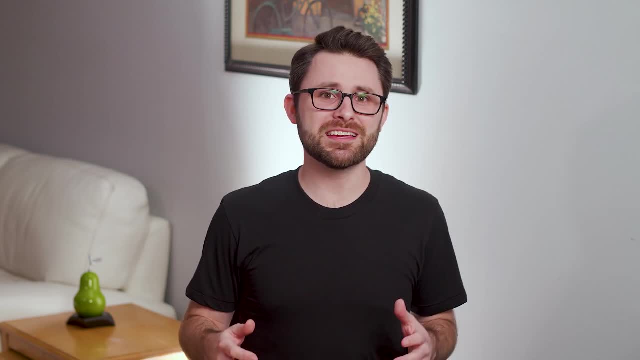 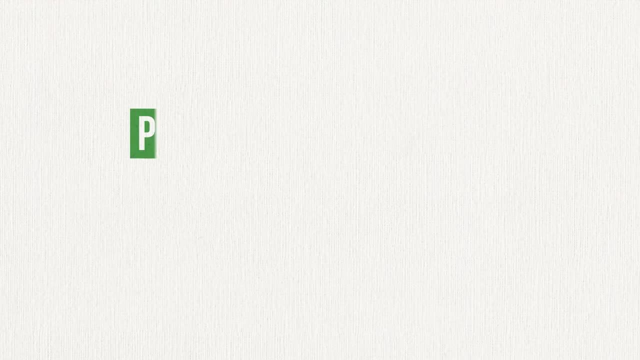 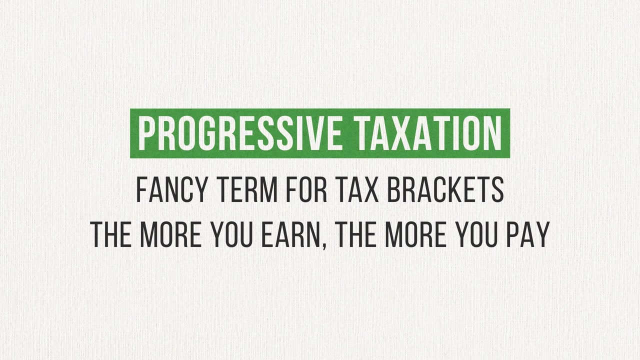 Because Uncle Sam is hungry. Two of the most important things to know about taxes are how progressive taxation works and how to file your annual tax returns. Progressive taxation is a fancy term for tax brackets. The more you earn, the higher the percentage of your income you need to pay the government. 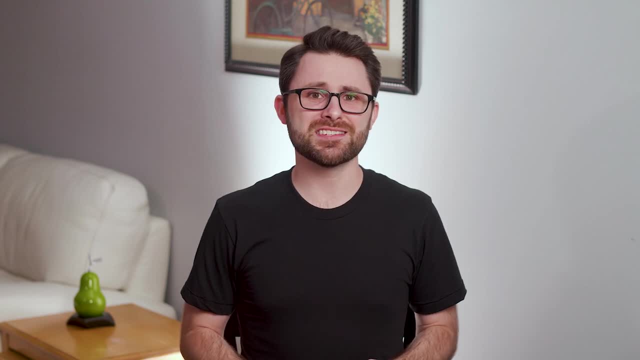 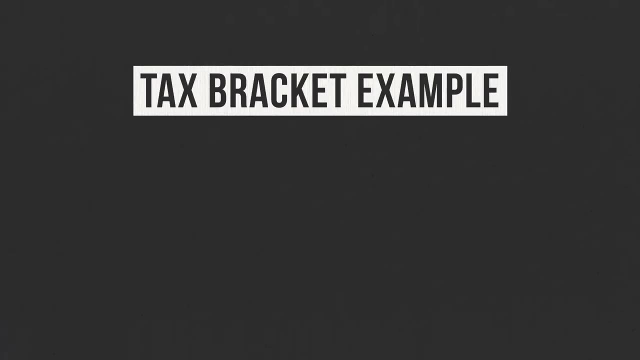 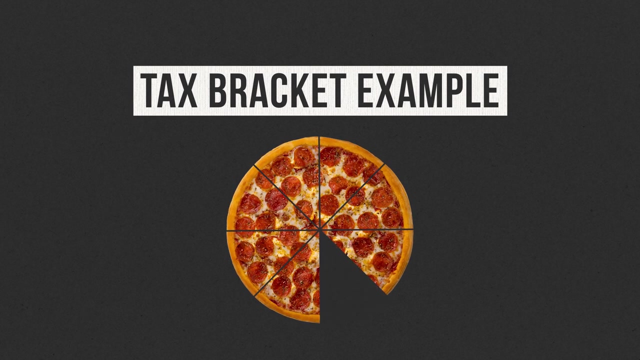 in taxes. On the surface, it's a pretty simple concept, But there's a major misconception. There's a misconception about how tax brackets actually work. Let's again pretend that pizza is income. When you get a single pizza, you're in a one-slice tax bracket and it shows up with one missing. 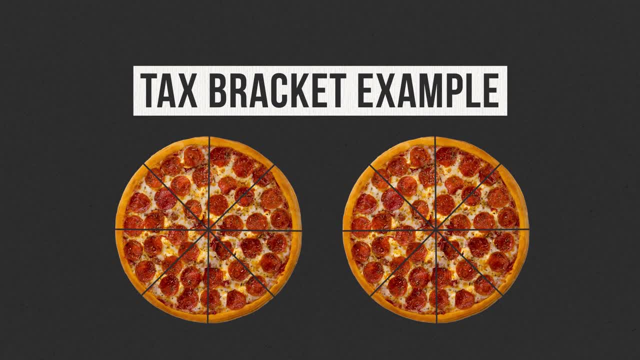 slice When you get two pizzas. now you're in a two-slice tax bracket. So how many slices would be missing in total? Most people mistakenly believe that each of those two pizzas will be missing. two slices for a total of four slices missing. 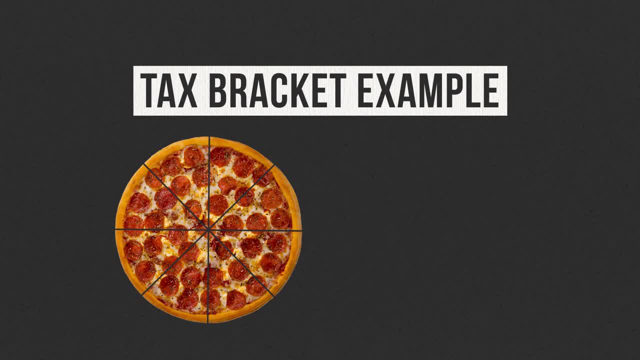 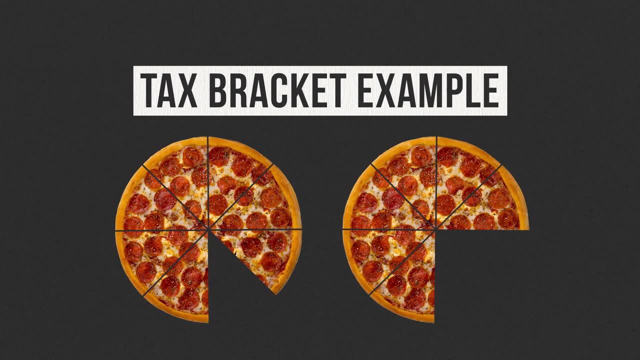 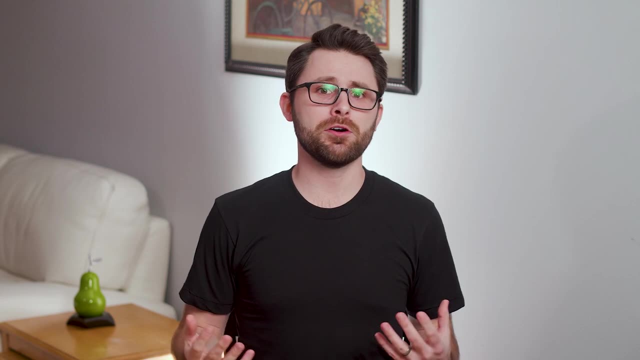 But this is incorrect. The first pizza will only be missing one slice, while the second pizza will be missing two slices, for a total of three slices missing. This is, in essence, how progressive taxation works. Filing your annual tax returns on your own is like a rite of passage when you become 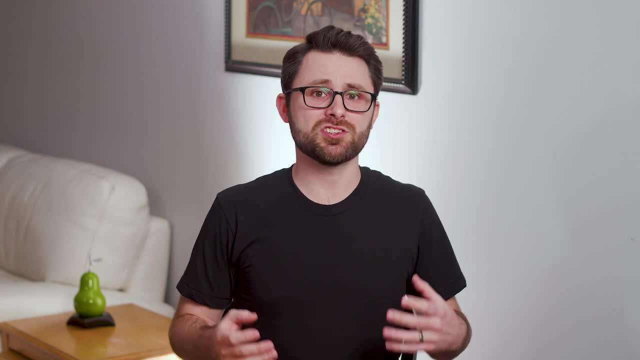 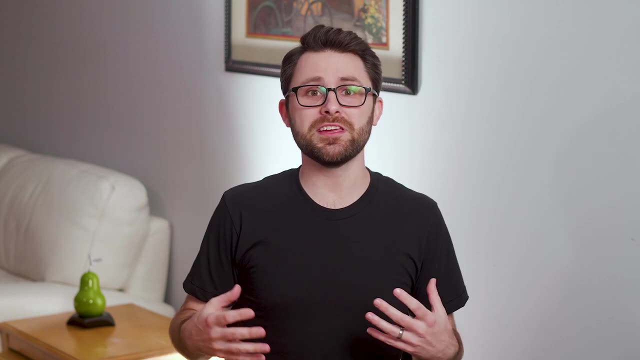 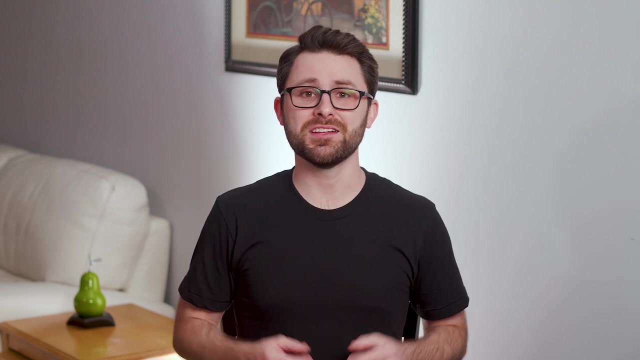 an adult, And if you're doing it for the first time, it can be a daunting task. Here's an overview of how it works. When your taxes are getting taken out of your paycheck all throughout the year, what you're really doing is paying the government an estimate of the amount of taxes you actually owe. 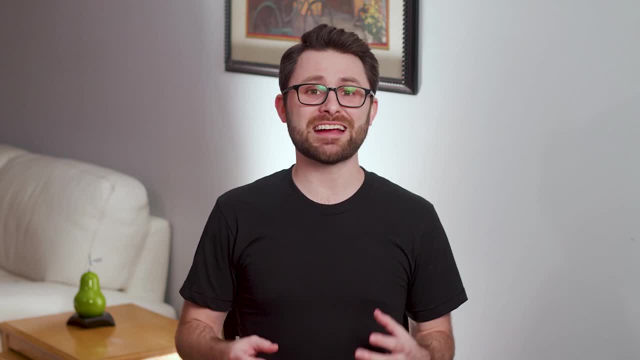 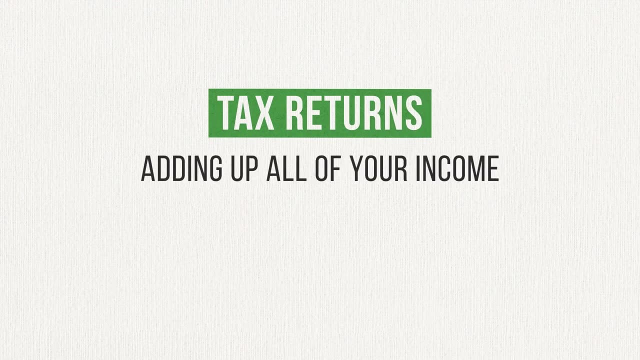 Until the year is over, there's no way to know for sure what your exact tax bill will be. That's where tax returns come into play. After the year is over, you're taking a look back, adding up all of your income and calculating. 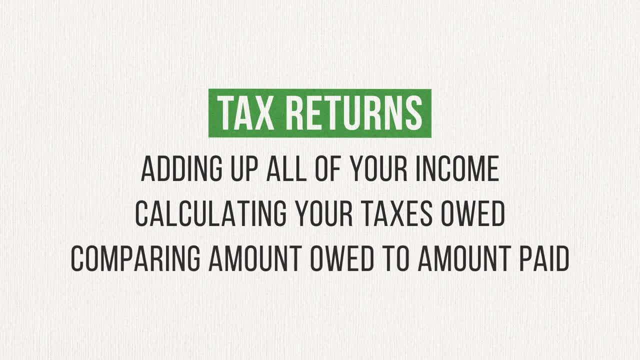 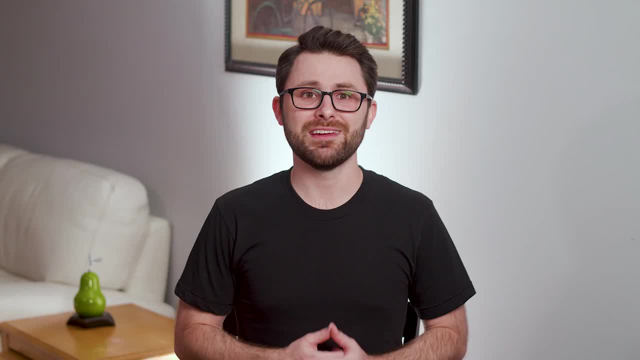 your taxes owed. Then you compare the amount of taxes owed with the amount of taxes you already paid. If you paid more than you owed, you get a tax refund. Thank you. If you paid too little, you need to pony up some cash. 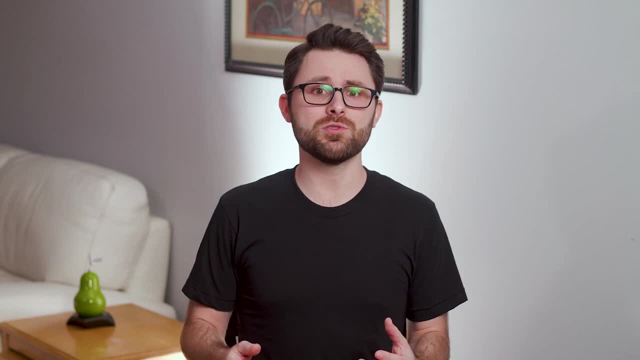 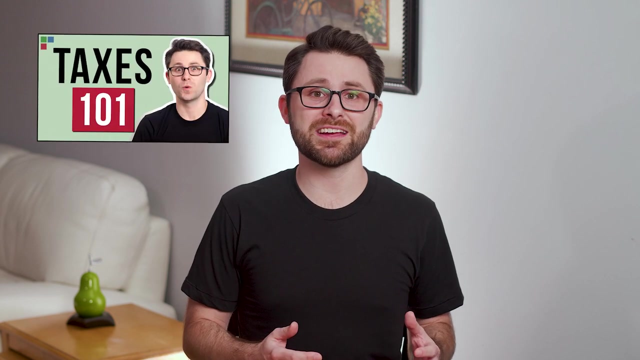 The tax return documents themselves are like worksheets that help you do all of the calculations, And there's no shortage of apps and tax professionals who will fill out and submit those worksheets for you. If you'd like to dive deeper into the topic of taxes, I made in-depth videos about how tax brackets work and how to file your tax return for the first time. 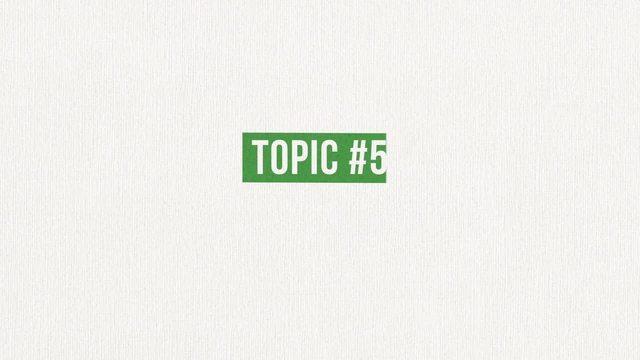 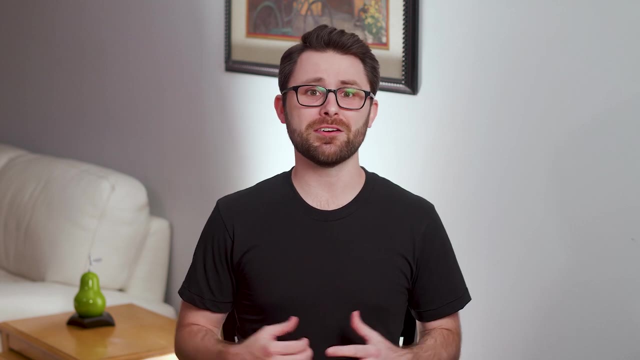 Links to both of those videos are down below. And finally, topic number five is credit scores. What if your best friend asked you to borrow some money to buy a new video game and promised to pay you back in a couple of weeks? If you had it, would you lend him the money? 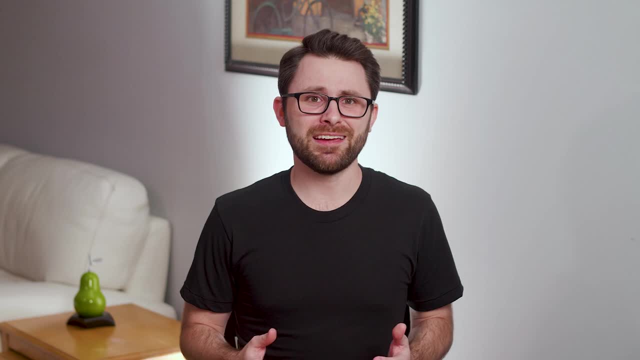 Sure, why not? You trust him, you see him just about every day and if he tries to stiff you, you know where he lives and you can get his parents involved. But what if a random stranger came up to you on the street and asked you for the same favor? 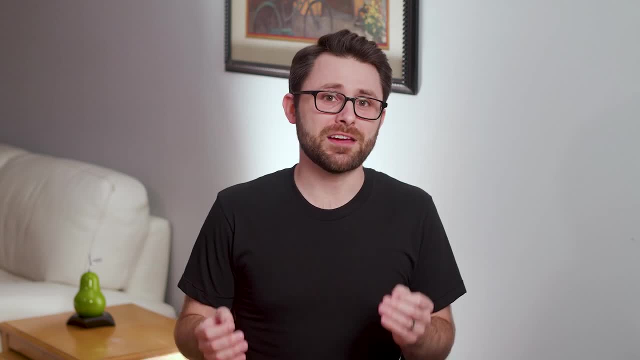 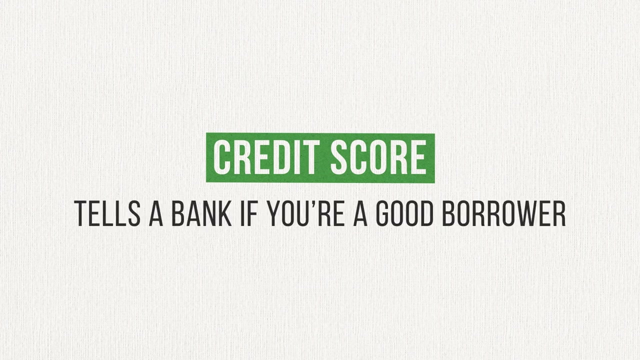 Would you do it? Of course not. And yet banks lend out huge amounts of money for houses and cars every single day. How can they tell whether or not that person is going to pay them back? Easy, their credit score. Your credit score is an easy way for banks to quickly determine how reliable you are as a borrower. 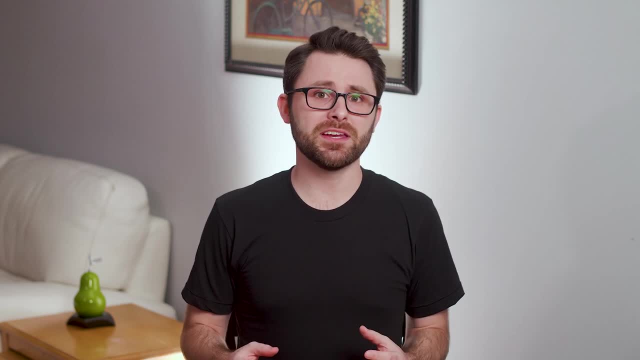 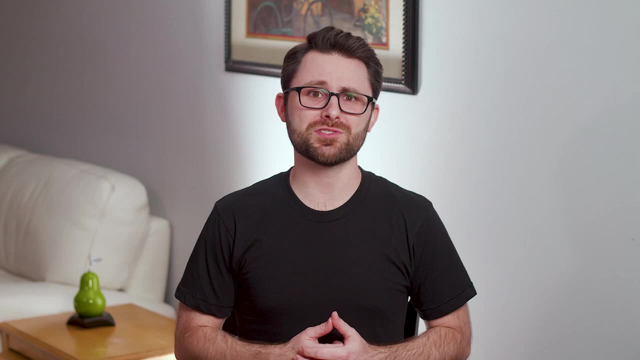 If you have a good credit score, it means you always repay the money you borrowed on time and in full with interest. Banks love lending money to people with good credit scores Because that's how they earn money and build fancy skyscrapers downtown. It's all those interest fees we pay them every month. On the flip side, if you have a bad credit score, it's generally an indication that you aren't a very reliable person when it comes to repaying your debts. Banks don't like lending money to people with low credit scores because odds are they're going to have to chase them around a little bit to get their money back. 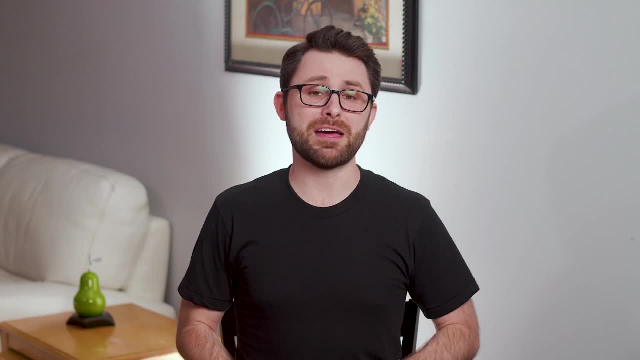 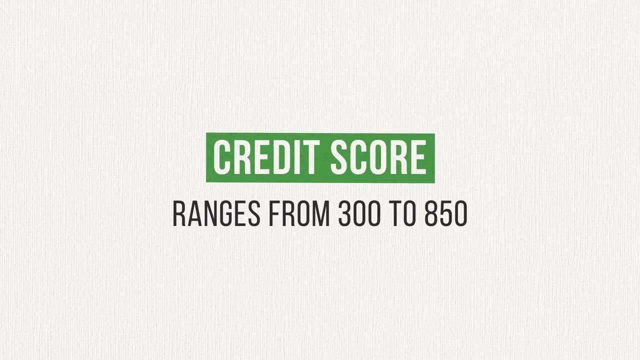 And there's a possibility they might not get their money back at all if that person vanishes or declares bankruptcy. Your credit score can range from 300 on the low end to 850 on the high end. Don't ask me why that's the range, it just is. 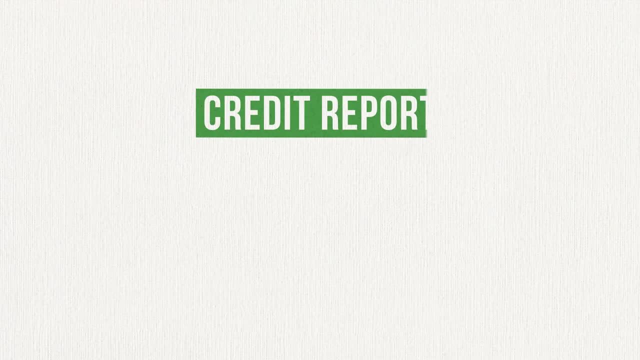 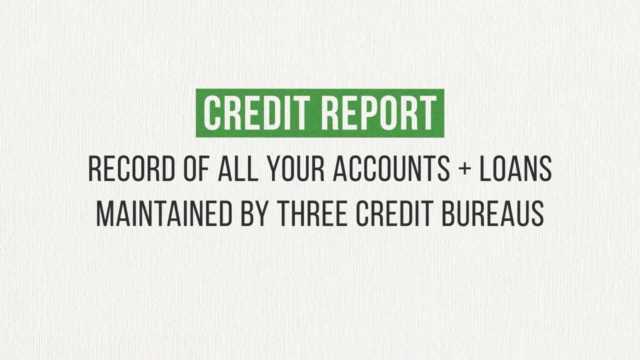 Your score is based on your credit report, which is a record of all your accounts, monthly payments and amounts you owe on loans and credit cards. This record is maintained by three independent agencies called credit bureaus. When a bank gets your credit score. 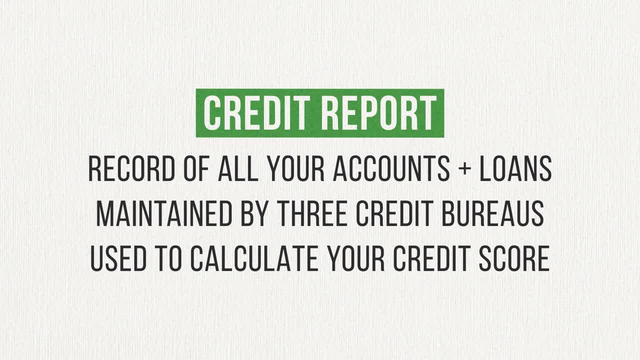 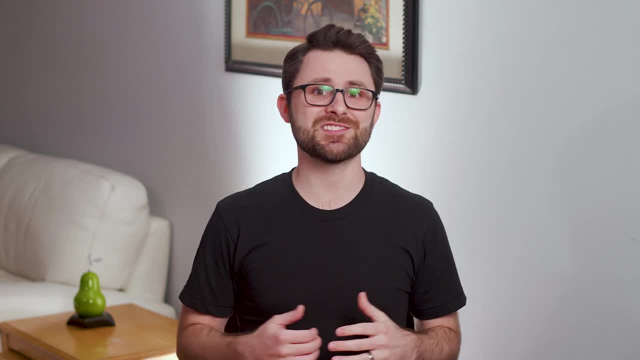 your record goes into a computer system that does some analysis and spits out a score, Just like how a Scantron form was fed into the machine and spit out a score for tests back when I was in high school. Are they still using those things? 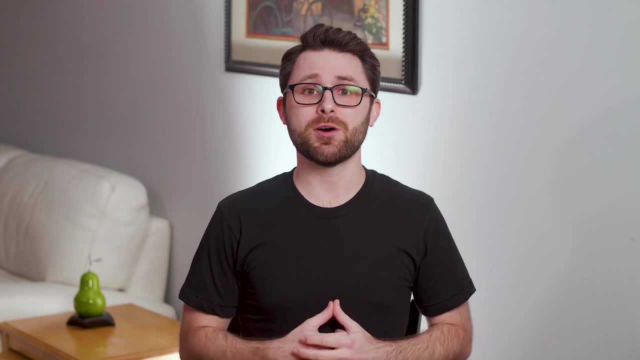 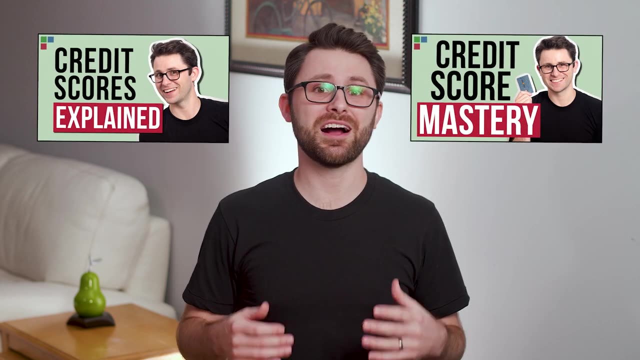 Anyway, if you want to learn more about credit scores, I recommend watching either my video about credit scores in general or my video about how to achieve a credit score of 800 or higher. Both of those links are down below. What else do you think a high school student needs to know about money? 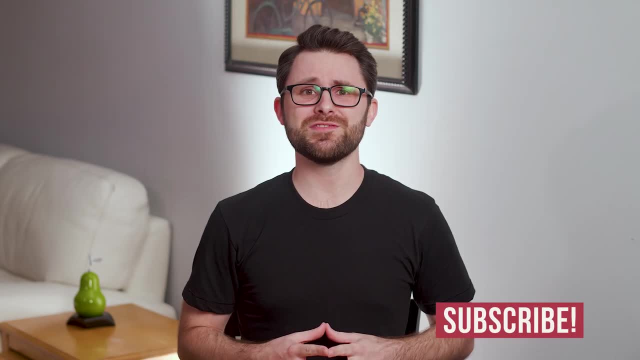 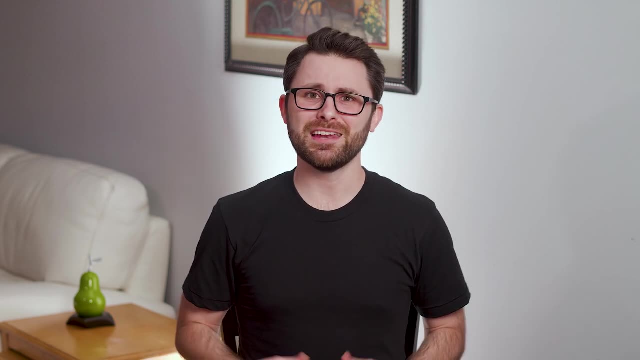 and personal finance. Let me know in the comments If you enjoyed this video. click right here to watch my video about how to set financial goals and why it's so important to do so, And if you'd like to show your support for my channel. 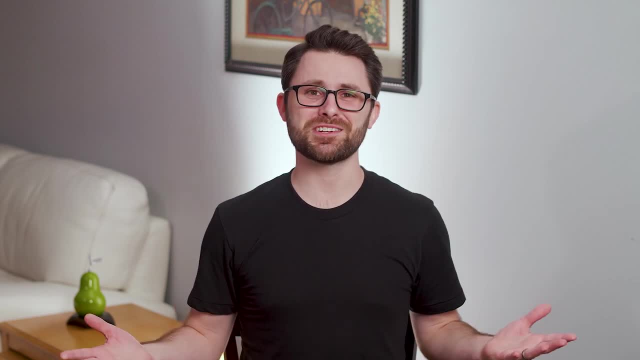 click right here to subscribe. As always, thanks for watching. I'm Andrew Scheer and I'll see you next time. 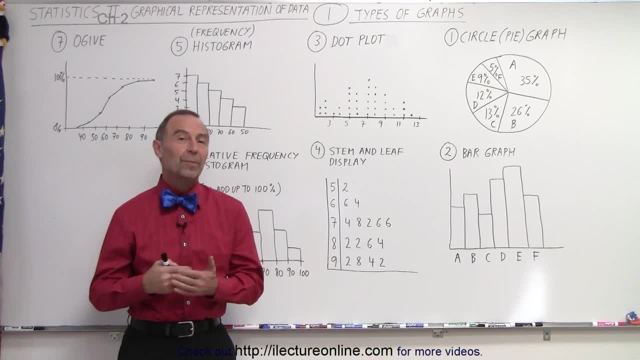 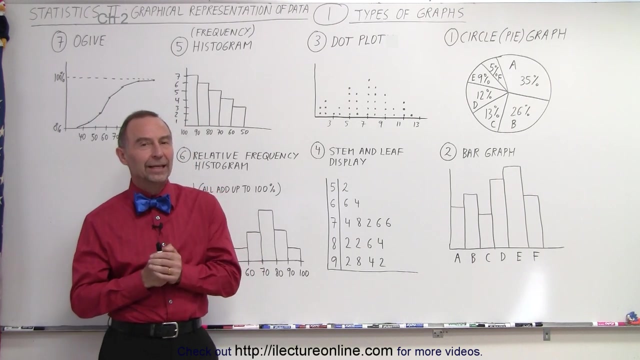 Welcome to iLecture Online. The second chapter in statistics is dealing with graphical representation of data. Well, it's collecting data, organizing them, graphing them and then interpreting those graphs. There's a lot of work to be done in this chapter and it all surrounds specific ways in 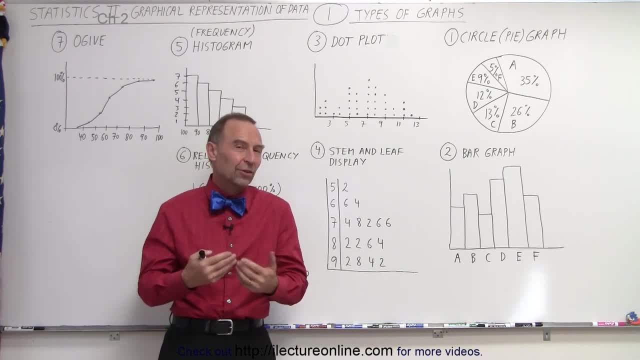 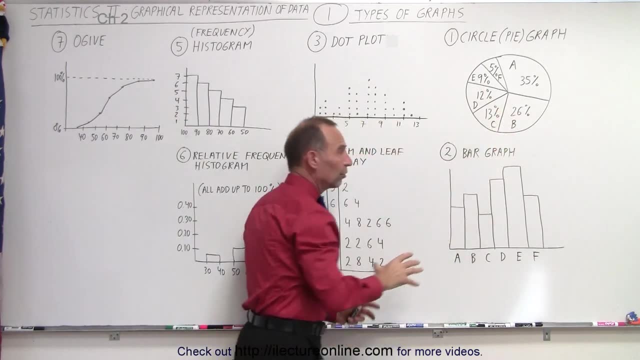 which we can represent the data. So here are some of the ways, some of the graphs that we will encounter in this chapter. First of all, we'll be encountering the circle graph, or also called the pie graph. So you can see that each slice of the pie represents a certain input of the data and you 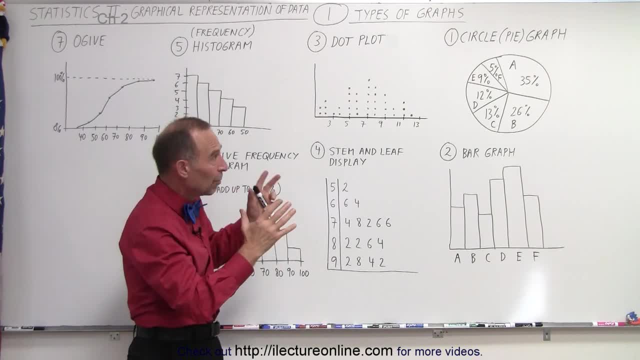 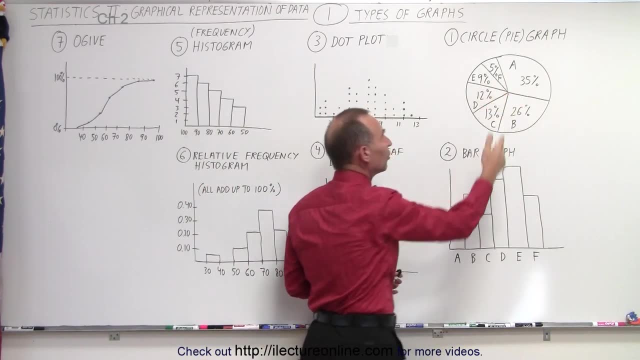 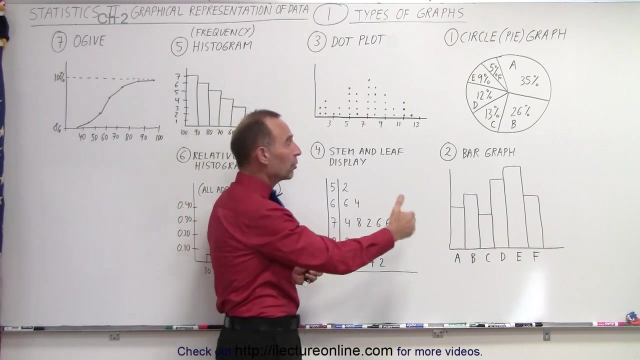 can see that typically the larger size of the pie means that more of it belongs to that specific data type. So here we have it generally labeled A, B, C, D, E, F, and you can see the relative percentages that each of those data types represent. Instead of the circle graph, sometimes we use the bar graph. 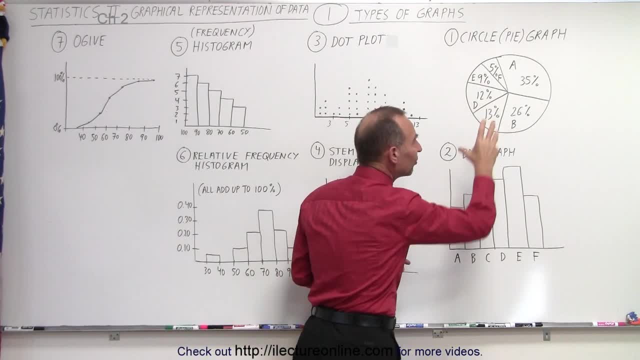 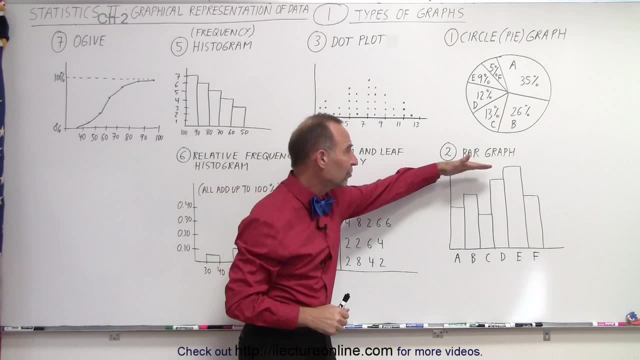 The bar graph gives you much more of a relative height. The sizes, especially when there's a lot of slices, are more important, So you can see that each slice of the pie represents a certain input of the data. The sizes in the pie make it sometimes difficult to see if one is bigger than the other. With bar graphs you can. 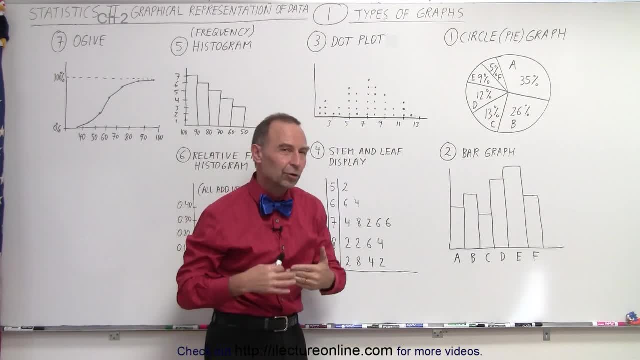 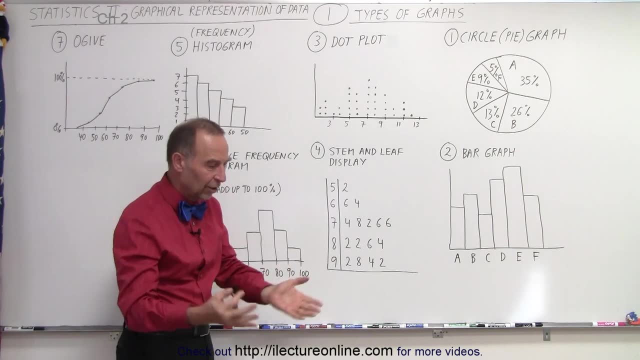 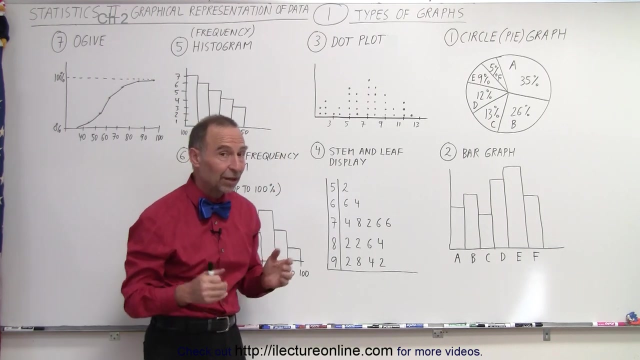 actually see very quickly which ones have the greatest height and therefore the greatest representation in the data set. We'll also encounter dot plots, which are very handy when you have a random set of data that you want to graph quickly. We'll talk about the stem and leaf display, which has some interesting aspects of it as well. 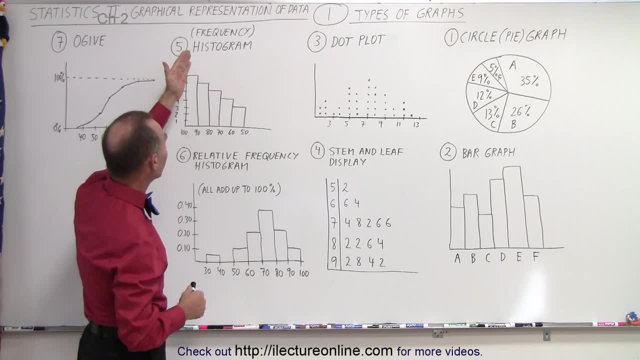 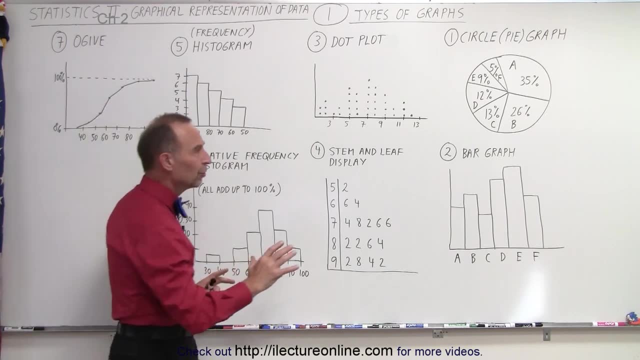 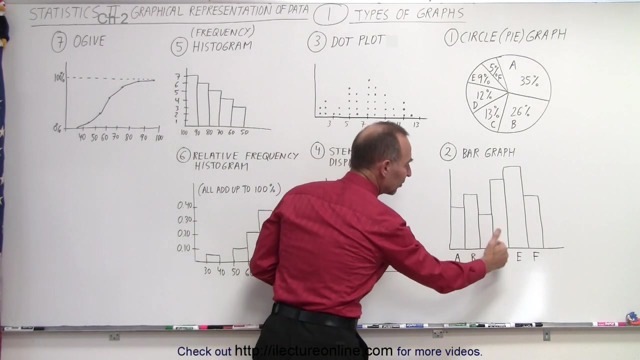 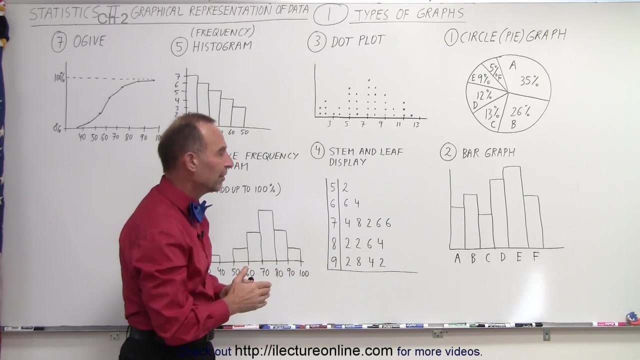 We'll also talk about the histogram. We have what we call the frequency histogram. A lot of times people get confused between the difference between bar graphs and histograms. Typically, bar graphs are associated with specific data sets. For example, if you have the number of types of cars, there's only one type of car of that type, and so you want to then see how many you have of each type.